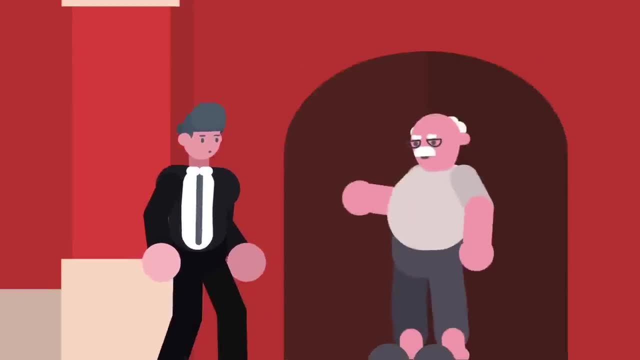 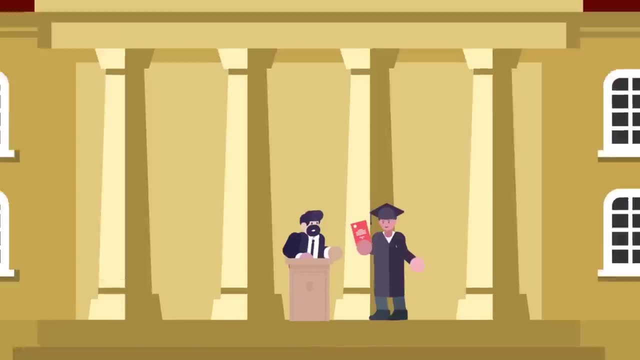 the youngest of people and that's because you have to put in some time first, as a teacher of nowhere might not be as stringent in hiring a principal for a primary school as an expensive private high school might be in a big city. when they hire a principal, Regardless, you're usually 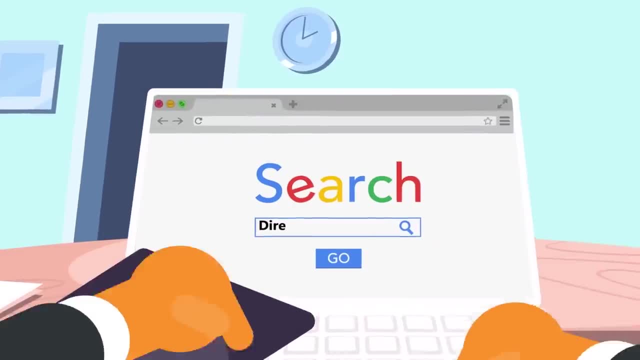 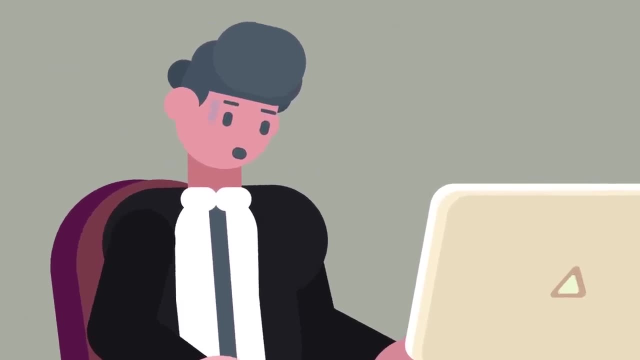 expected to have earned a bachelor's degree. We went to the job website, indeed, and had a look at job postings for principals, and we can tell the duties and responsibilities part of the job offer put us off right away. It seems some schools were looking for someone who might. 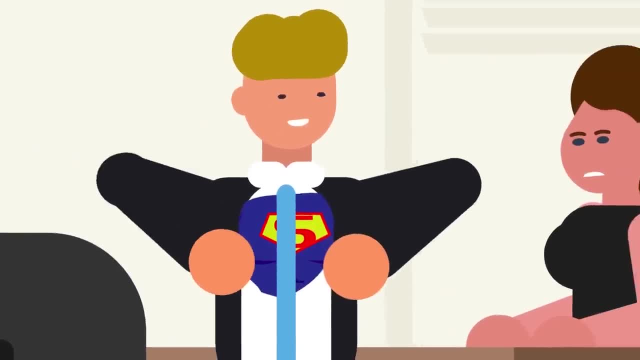 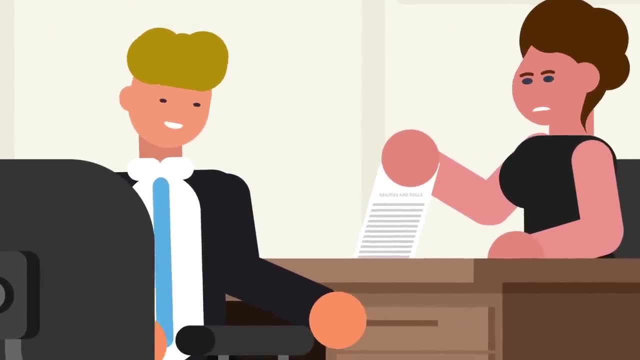 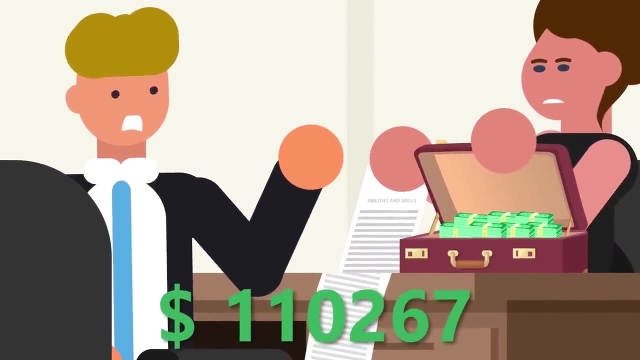 resemble something more like Superman than a school administrator. The list of abilities and skills and personal qualities required made it sound like they were looking for human perfection. but for at least one job we looked at at least, the pay was up to $110,267,. so that's not such a 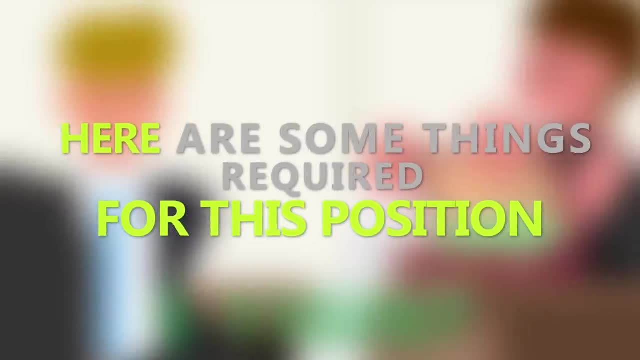 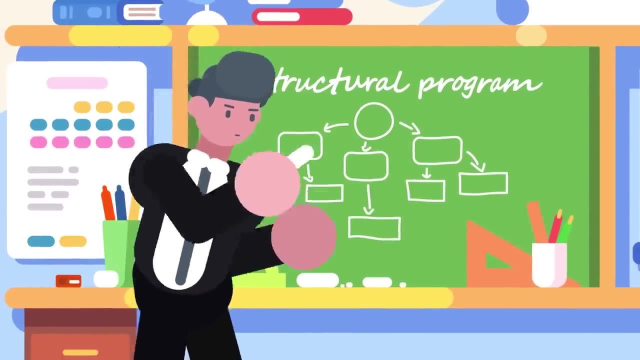 bad amount once you've mastered everything. Here are some things required for this position. You must have success in philosophy, curriculum and instruction. You must know all kinds of instructional strategies. You must have a good sense of the world. You must have a good sense. 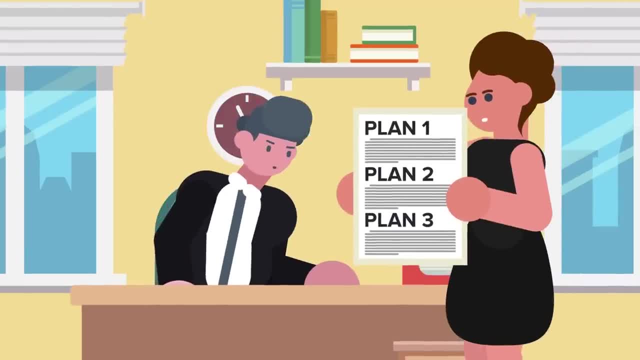 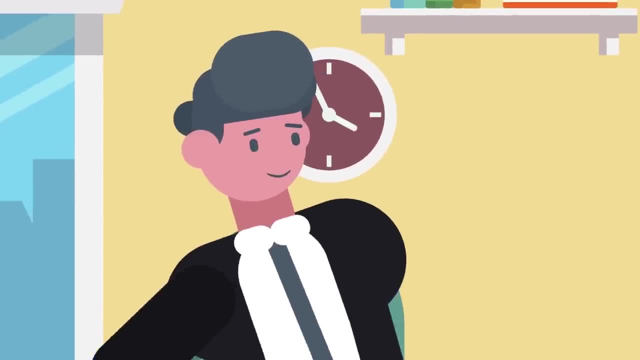 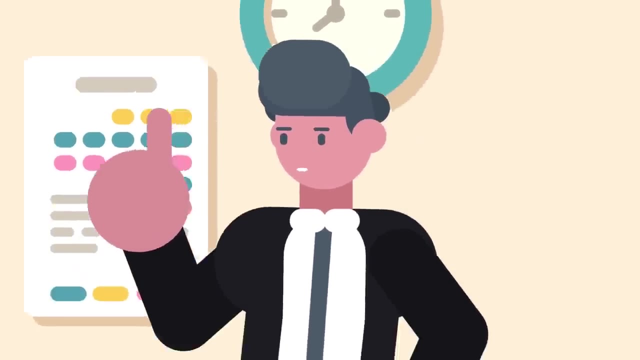 of strategies and improve structural programs. You need to be effective in planning, allocating resources, scheduling, finding logical conclusions and making good decisions while using appropriate decision-making processes. You need to know the latest education-related computer tech. You must have great judgment, formidable insights, while exercising self-awareness at all times. 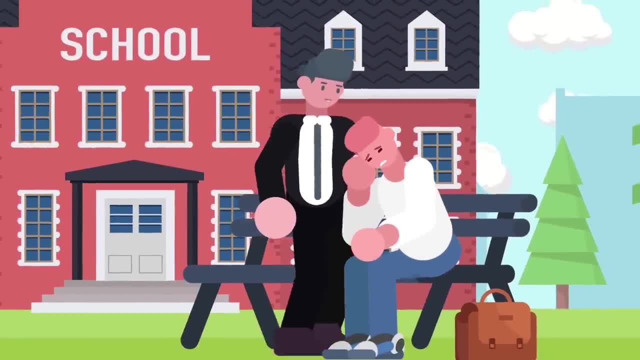 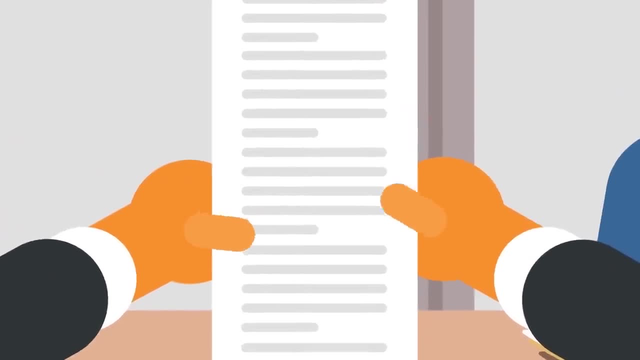 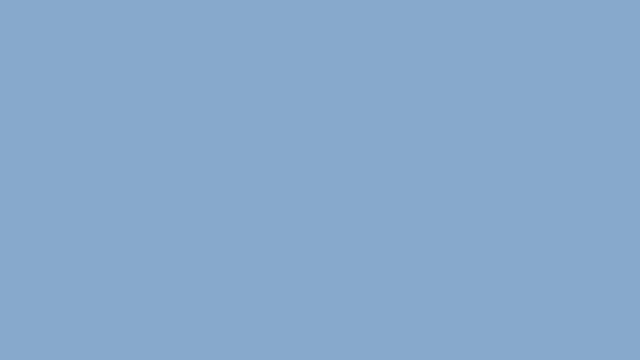 And these are merely a few in a long list of attributes required to get that job. But in terms of academic qualifications, yep, they all asked for that bachelor's degree. That's pretty much right at the bottom of what you'll need, Like saying, a brain surgeon will. 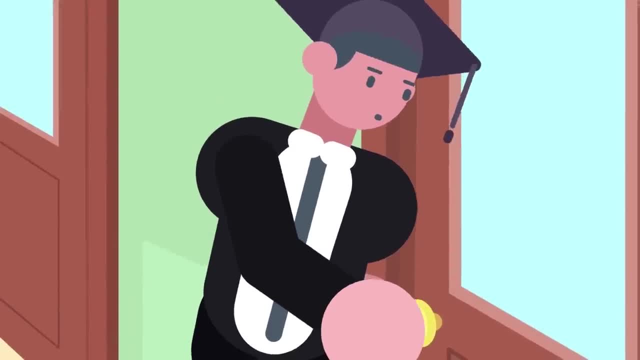 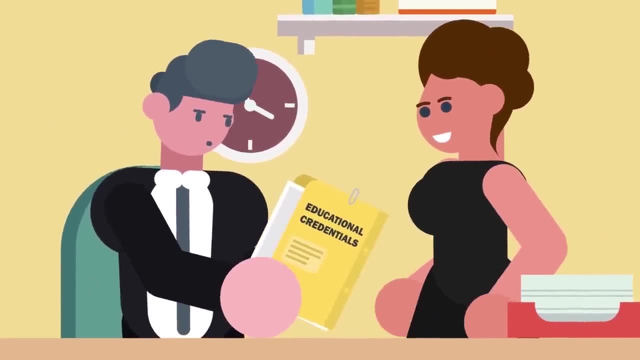 need eyes and hands And a brain. After that, some places will require that you have a master's degree, but not all. You'll also need some kind of teaching credential, which differs from country to country. In many places, you'll also need an administrator's license, which will require a master's degree, But, as we said, this can change depending on where you teach. You'll need teaching experience, then some administration experience, but how many years differs from school to school. One job we found asked for at least five years teaching experience and three years admin. 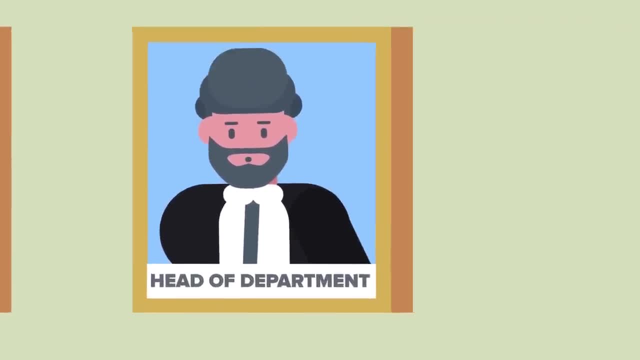 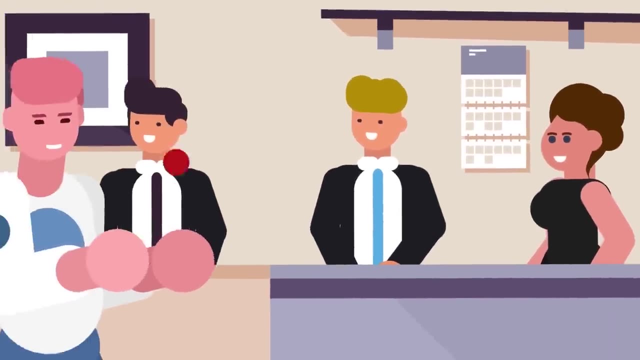 experience. Many principals have been heads of departments for years before they climbed up through the ranks to the big boss chair. So you've demonstrated you have more skills than any human is actually really capable of, and you have the certificates and experience. You, in my opinion, 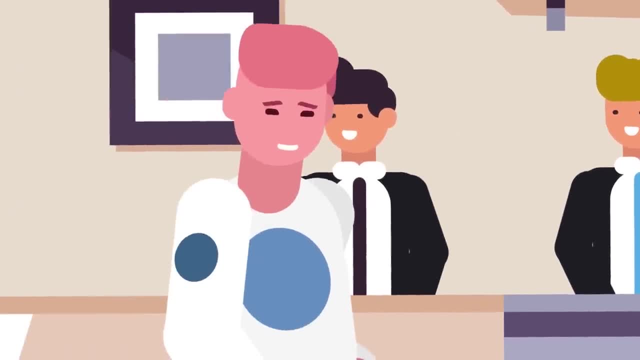 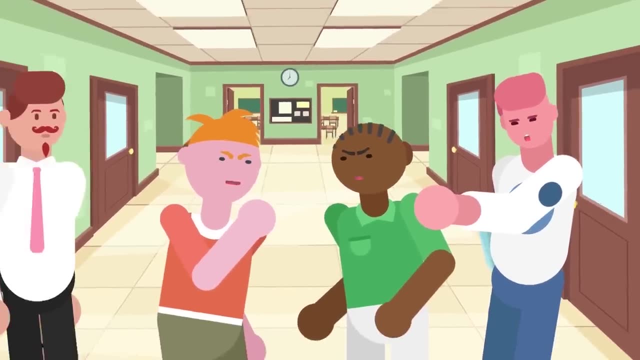 impressed the interview and you have the job. Ok, what are you expected to do? Well, before you even reprimand your first student for fighting in the hallway, you'll have to know a lot about the philosophy of teaching, sometimes called pedagogy. You'll have to be fluent in various instructional 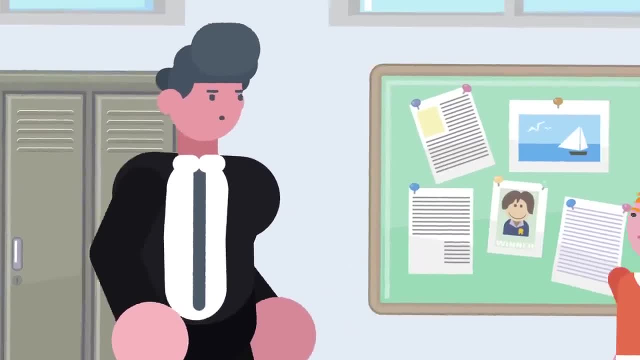 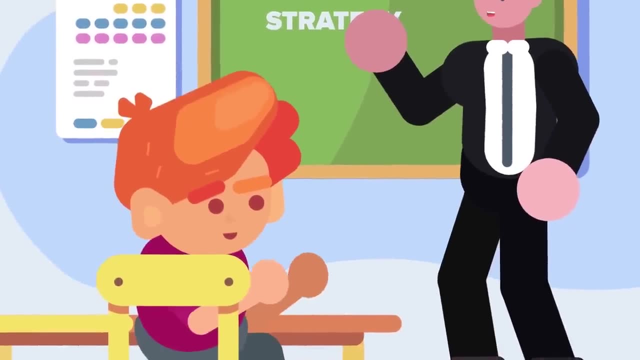 strategies and how to understand data. You'll be cool-headed and responsible, knowing how to get the best out of your teachers and students. You'll have strategies to get both teachers and students through the curriculum. You'll apply your strategies to meet the standards. 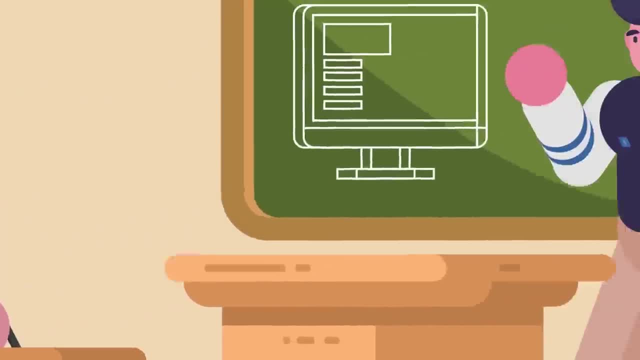 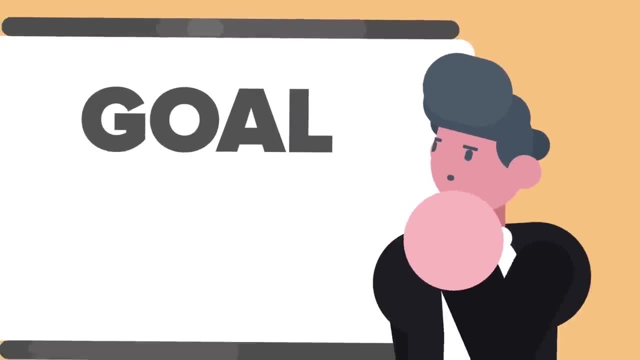 of the curriculum, You'll also understand various computer technologies related to teaching and admin. Let's say you know all that, What about your job day to day? Well, there's the goal and there's the daily operations. The main goal is to implement curriculum standards set by the 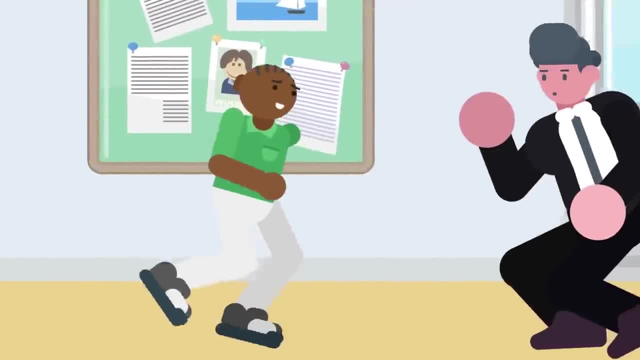 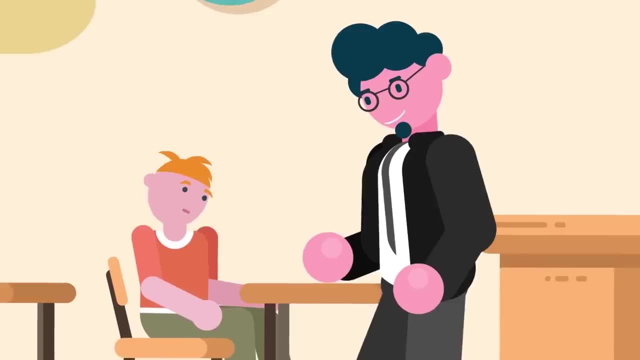 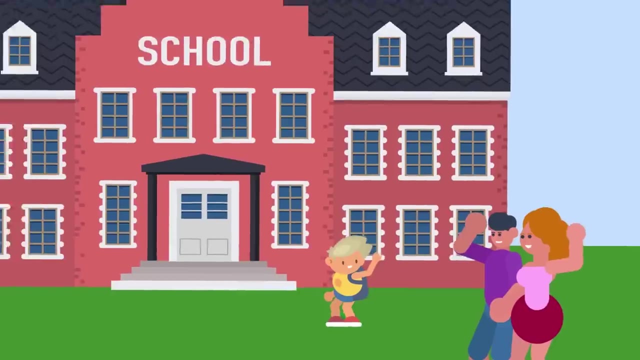 governing body in a district or country. The day-to-day job is that you manage the school, the teachers and the students. Your target is to get people through school with good grades and that in turn makes the school look good. If the students are getting straight A's, something is going right and parents will want to send. 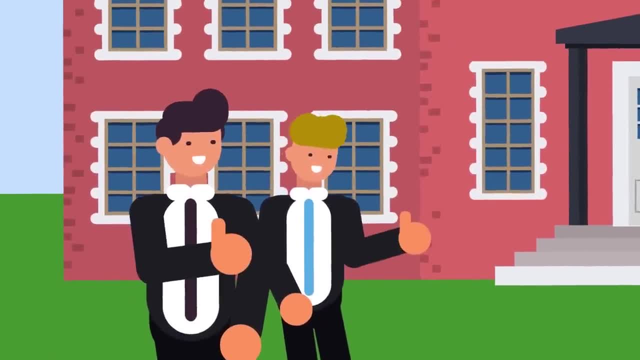 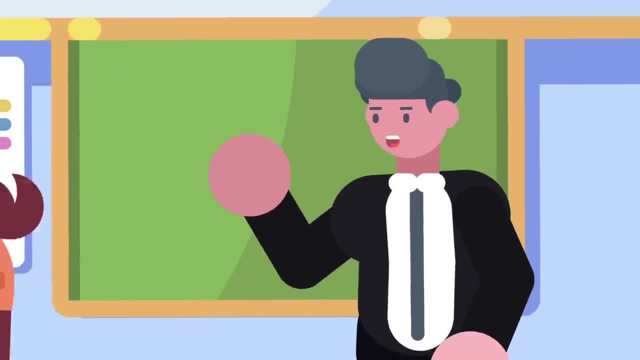 their kids to that school. The school gets a good name and the principal can bask in the light emitted from his computer monitor. He doesn't get out much, But another important aspect of this management thing can be a little bit like coaching. Ask any teacher how many meetings they have to. 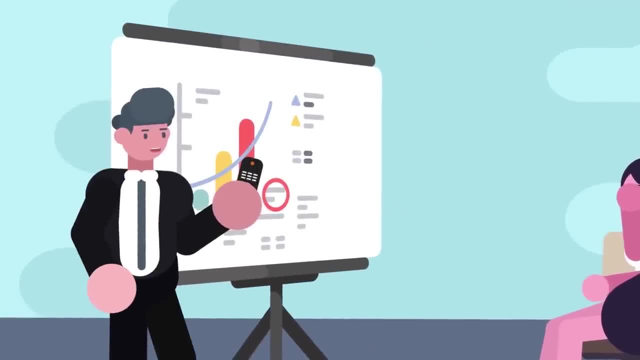 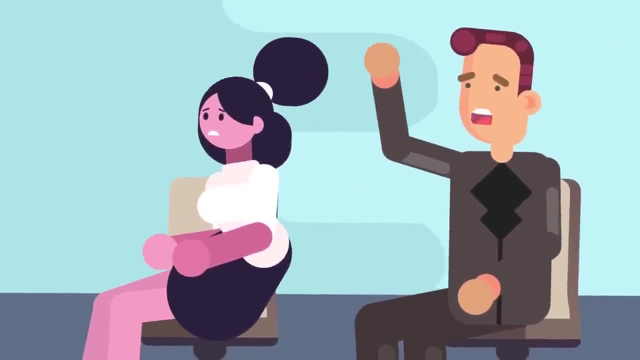 attend, in which the principal tells them about goals, usually with the aid of some PowerPoint slides and some jokes he thinks are funny. There will be coffee and cake too, which is always a bonus after a three-hour instructional marathon that keeps getting interrupted by teachers putting. 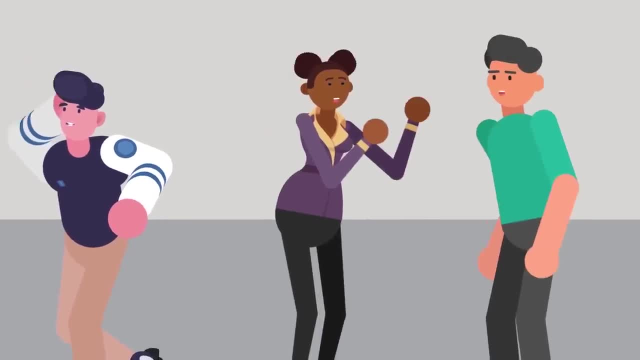 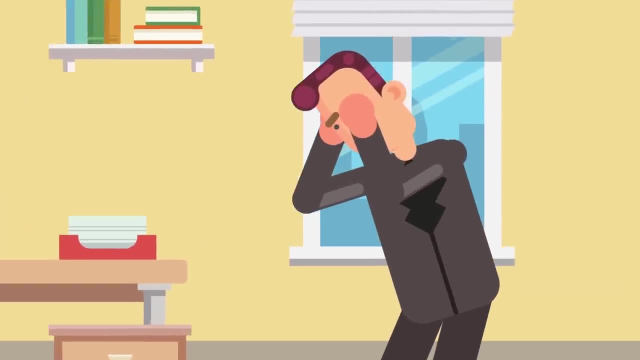 their hand up. That coaching is also done in the principal's office and there's usually a queue of people wanting to see this person. She won't go a day without hearing a complaint from a teacher or having to tell a teacher that they need to improve somehow. The same goes for students. If a 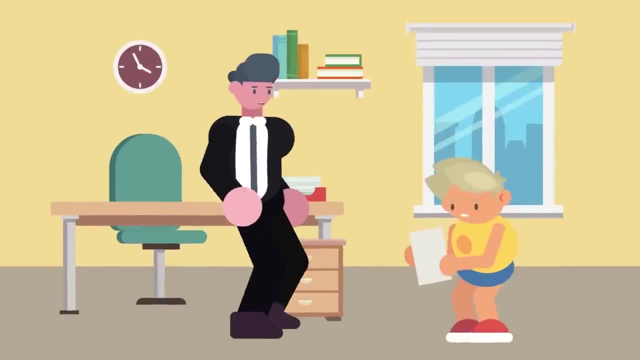 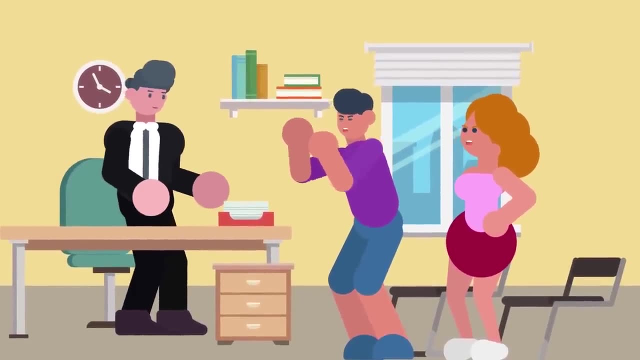 particular student is troublesome or lagging behind, he might have to visit that office for a bit of coaching, If that isn't enough. he'll also be in almost constant talks with parents who are just curious about their child or are annoyed about something related to their child's. 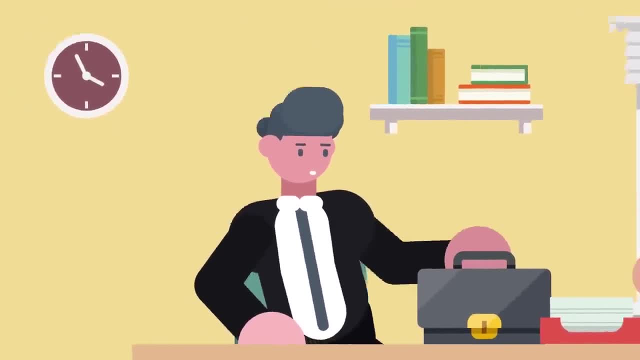 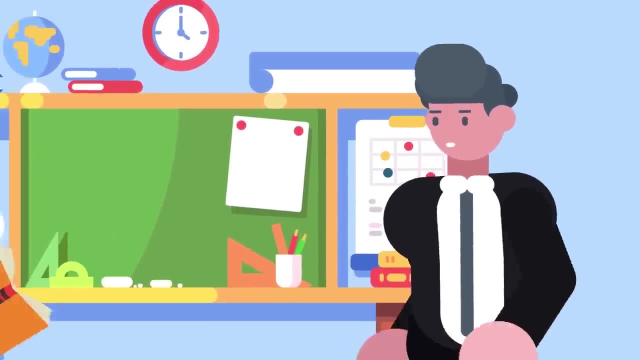 education. That's quite the job in itself, but we're not even close to finishing. A principal will also do workshops, observe teachers now and again and just walk around and see how things are going. He'll attend events such as concerts or sports games. She'll make sure the school is. 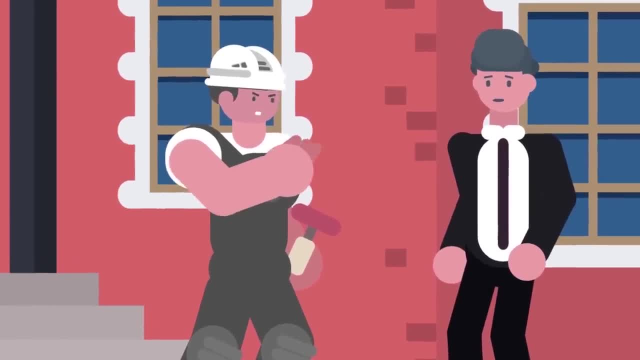 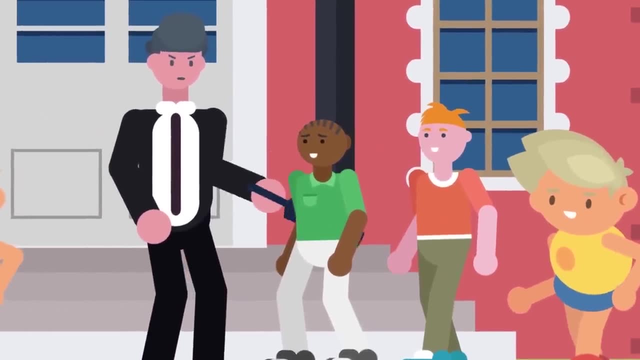 properly maintained and in many cases will have to figure out the budget for the huge amount of services and supplies the school needs. He must ensure the school is secure and safe for kids, for teachers, for visitors. He'll know the security guard, if there is one. 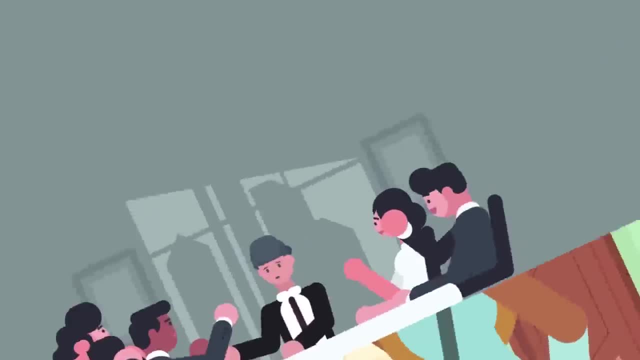 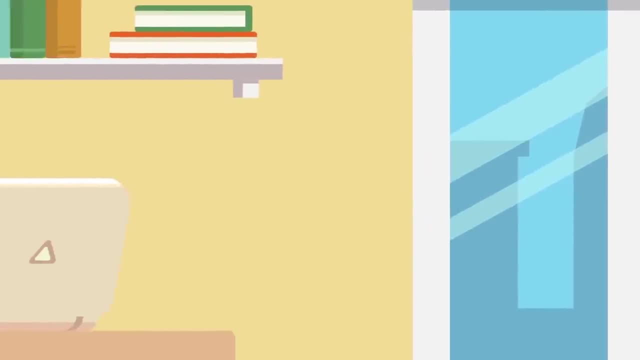 by name. She'll likely get along with the cleaning staff. He's the face of the school and so he'll also have to know the community, the people who fund the school, the legislators. This already sounds like too much, but, as we said, they are expected to be walking perfection In. 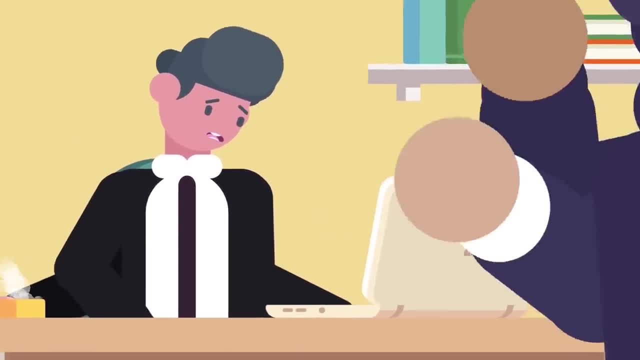 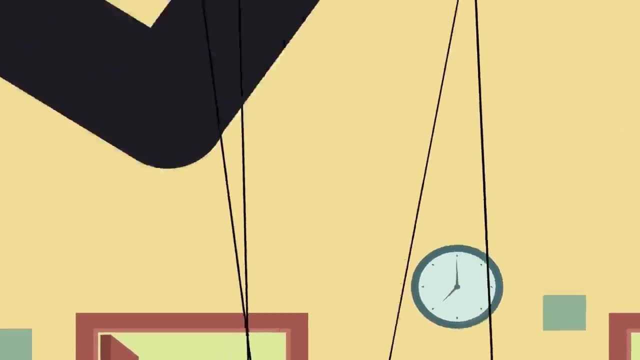 some schools this can be too much, even for a super principal, so he'll have an assistant principal. Heads of the departments also help to lessen his burden, but in the end they all report to the principal. The job doesn't usually make the 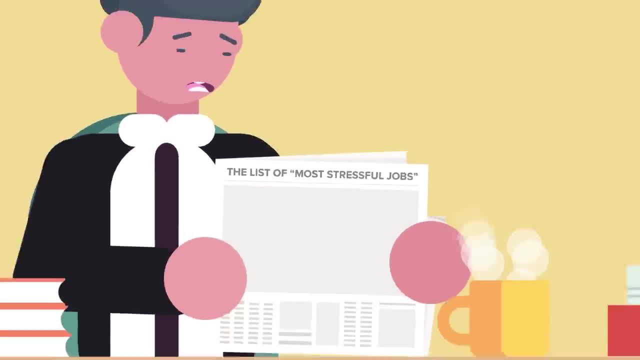 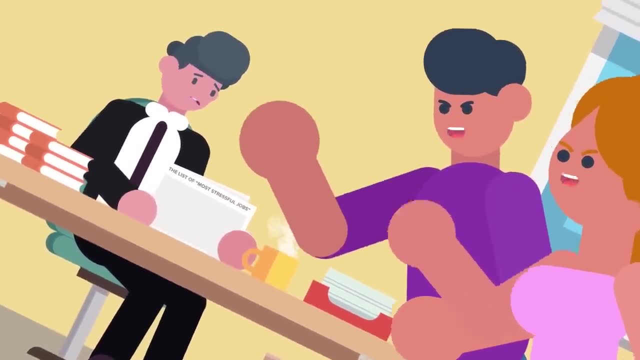 list of most stressful jobs, but it can be very stressful, especially if academic standards aren't being met or parents are constantly screaming at you or one wayward student just punched you in the face. This can happen, but some principals have gone into schools that were chaos and turned. 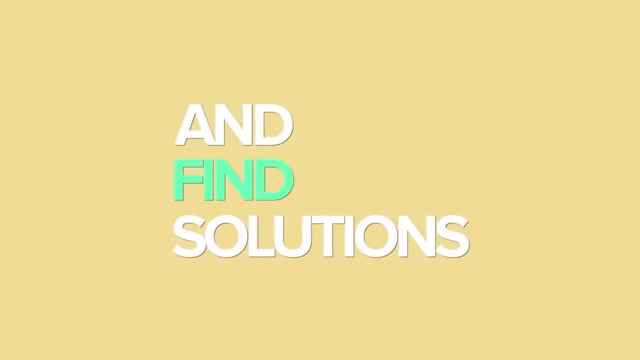 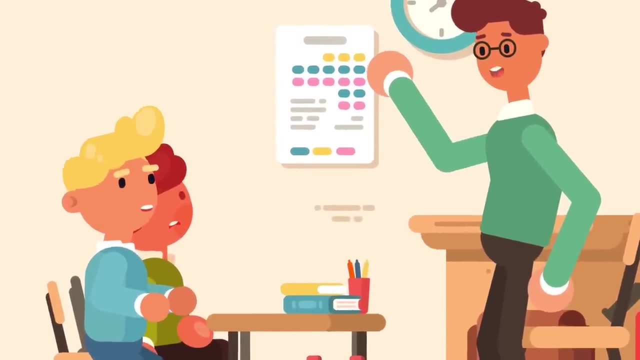 things around. A real super principal can assess problems and find solutions. Let's say that a principal has a student who has been referred to them because of discipline problems. This might in some cases be little kids lashing out in the classroom, but it might be much more serious. We all know that teachers have been attacked in the past. 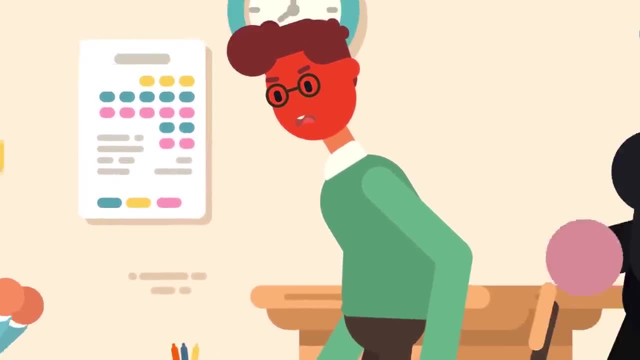 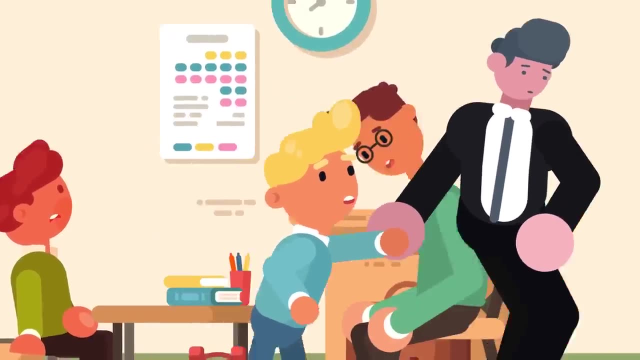 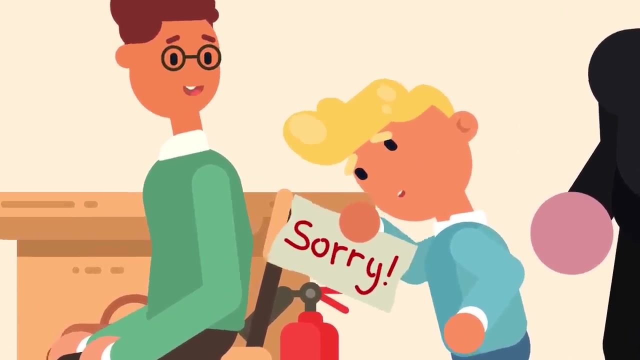 and this happens pretty much everywhere at some point. This is where the principal becomes the counselor, the mediator, knowing how to be stern but also knowing or trying to know why this student is problematic. If that principal can gain that student's trust and help encourage him or her to do and be better, then that principal 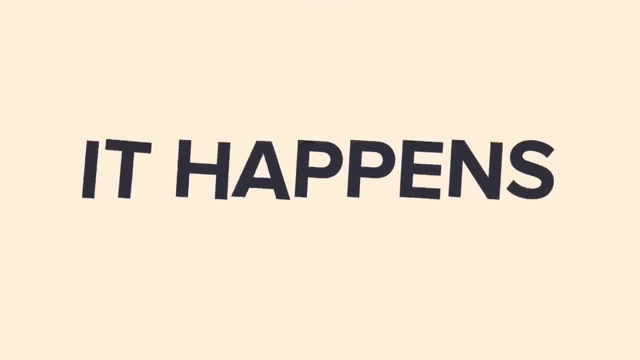 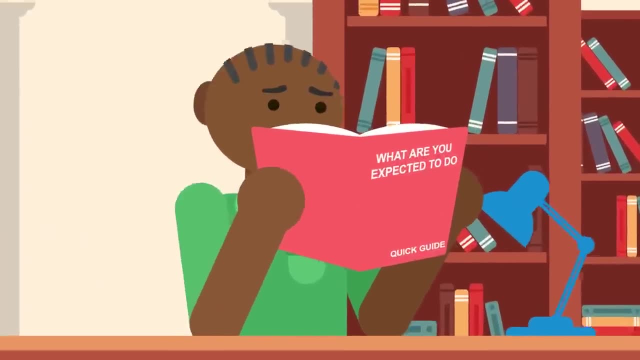 can help support them. Sometimes the kids just have to go. It happens If disciplinary action is taken. the principal should be fair. Students, on the other hand, have to know how they are expected to act and what they are expected to do. The principal might look at school policies and 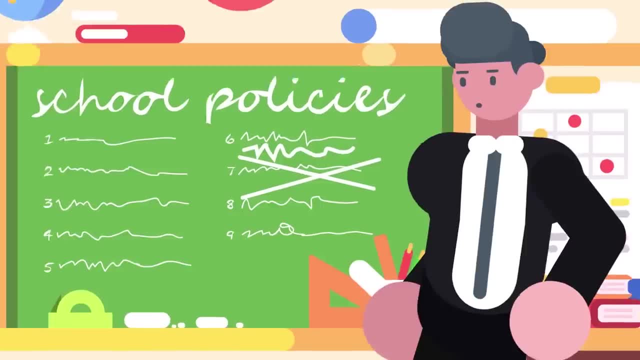 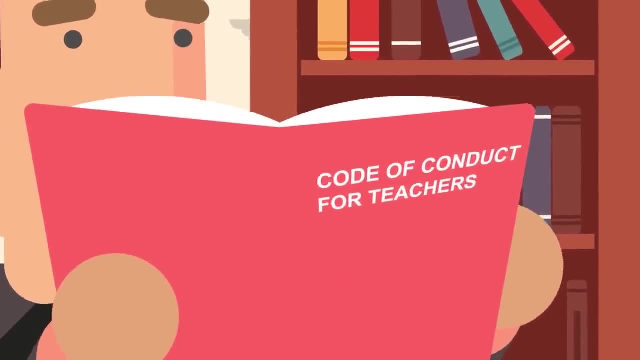 update them totally, rewrite them or create new policies and rules. The teachers, too, will have a code of conduct, and they can be fired or not, get a new contract for the next school year. They will also have a handbook. They could find themselves in the principal's office for not. 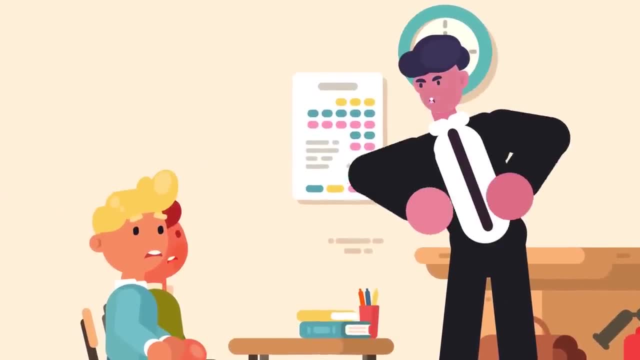 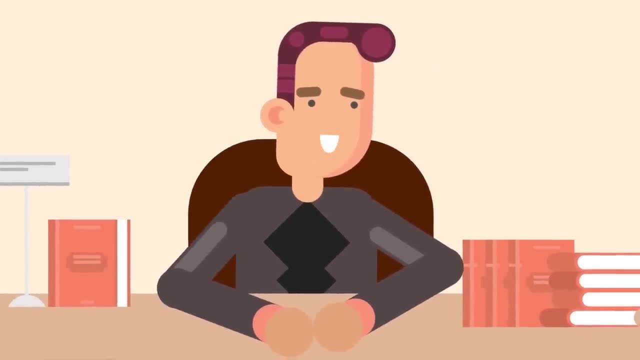 the dress code, or for using bad language in class, for not getting the right results, perhaps even for losing their temper in class. If a teacher is let go, a new one will have to be found. The principal will assist in finding that new teacher and he will likely have the. 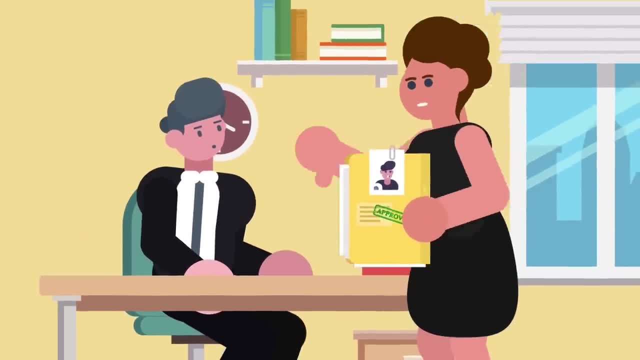 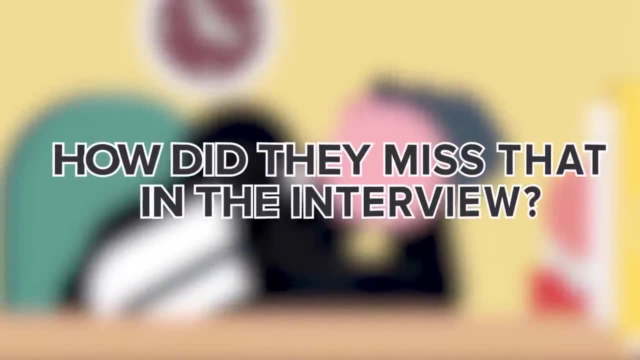 last say after the interview. This can also be stressful, because if that teacher turns out to be a bad hire who breaks rules, then that also comes back on the principal. How did they miss that in the interview? This does take a special person to do the job and not all people are up. 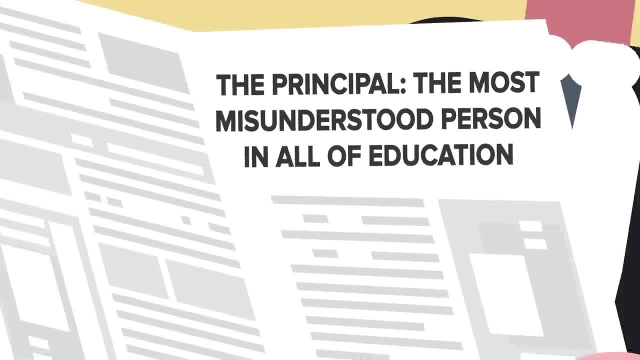 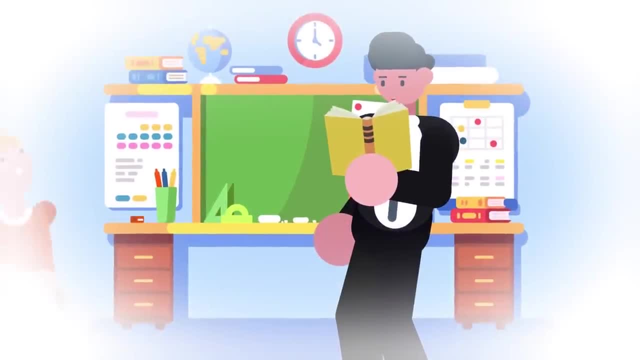 to the task. In an article in The Atlantic, the writer called the principal the most misunderstood person in all of education. It's said most people think this person spends all day lecturing students about using bad language and dealing with soppy or melodramatic or overly. 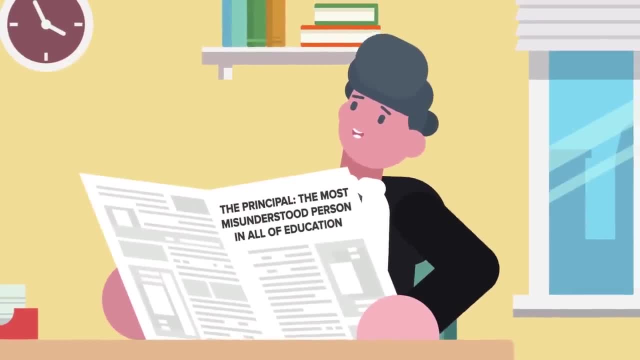 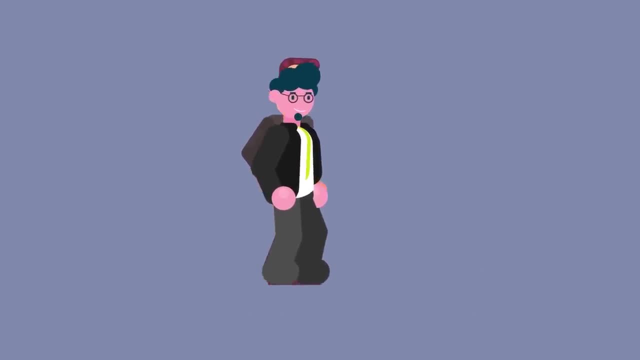 hostile teachers. But no, they spend much of their time dealing with the bureaucratic education system. The article said the principal is both the administrative director, director of state educational policy, and a building manager, both an advocate for school change and the protector of bureaucratic stability. 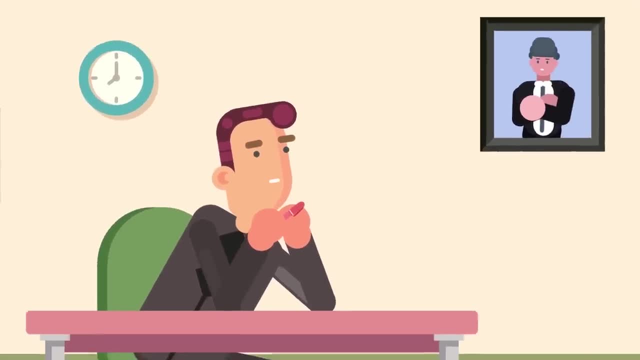 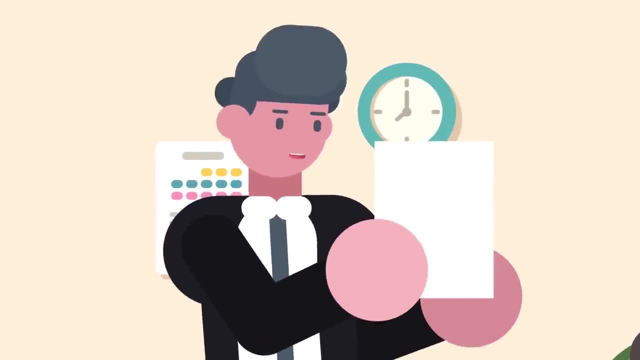 They're supposed to be an inspiration to all, a cornerstone of righteousness. not only understanding the latest in teaching methods and ensuring standards are met, but they have to get a grip with things like youth culture. It's true, kids will have more respect for a principal who knows what they are about. 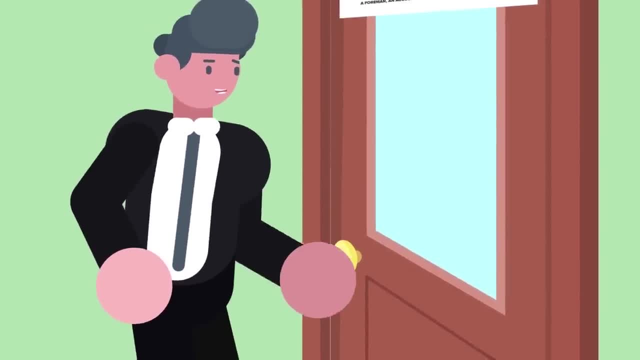 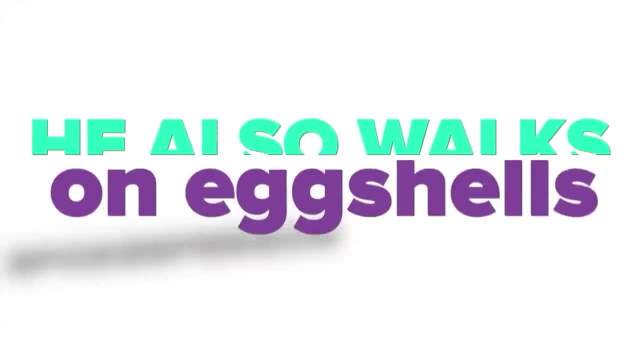 and where they're coming from. He's a middle manager to the powers that be a foreman, an accountant, A researcher, a spokesperson and an expert of the ever-evolving culture of the young. He also walks on eggshells. It might be fine for the local artist or truck driver to go out and